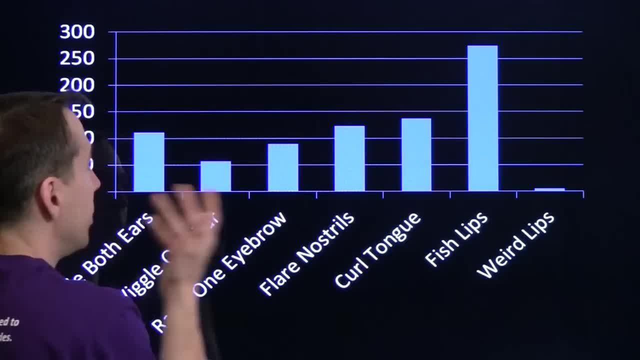 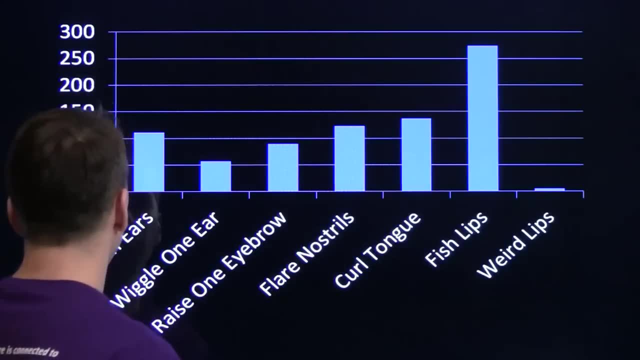 to be a real freak to be able to do that. Now you can also compare all any two of these. You can quickly see: Curl tongue- that's easier than wiggle one ear. Flare nostrils- that's easier than wiggle both ears. We can put them. 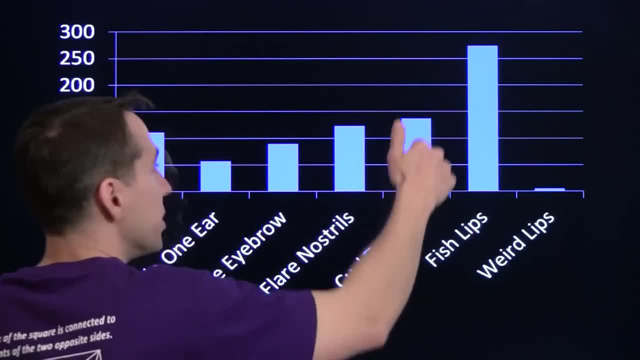 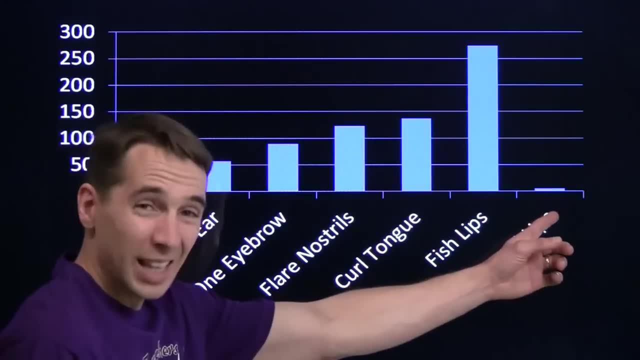 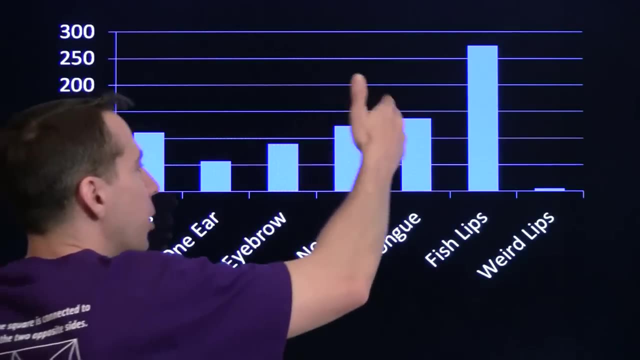 in order just at a glance: Tallest bar fish lips, Next is curl tongue, Next is flare nostrils, Next is wiggle both ears, Then raise one eyebrow, Then wiggle one ear And then last the hardest weird lips. So the bar chart here allows us to compare pairs very easily. We can see: 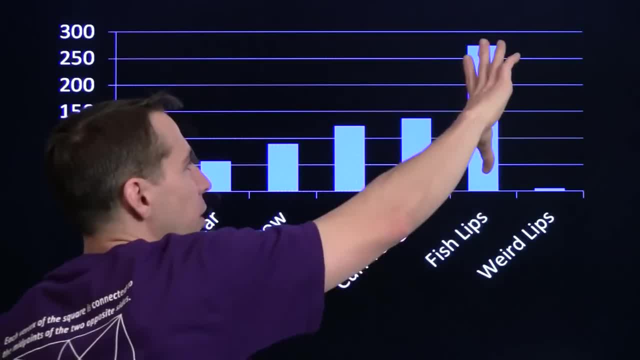 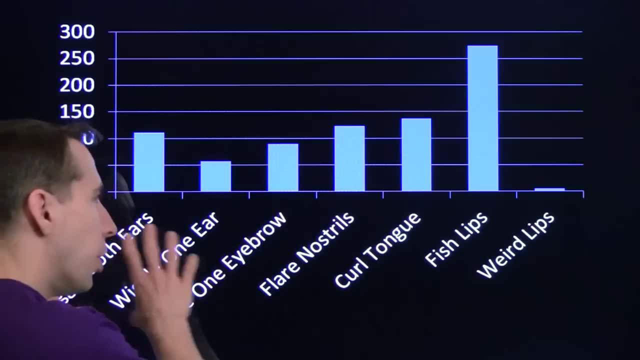 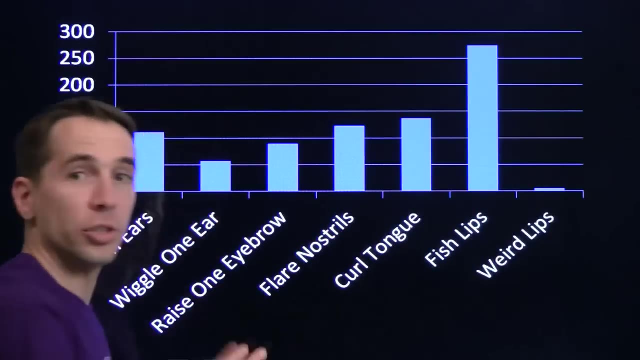 we can see the relative comparison too. See, fish lips is about, you know, on the order of twice as common as these, And it's just way, way easier than the weird lips. So the bar chart gives us a nice graphical, quick glance way to compare different skills to. 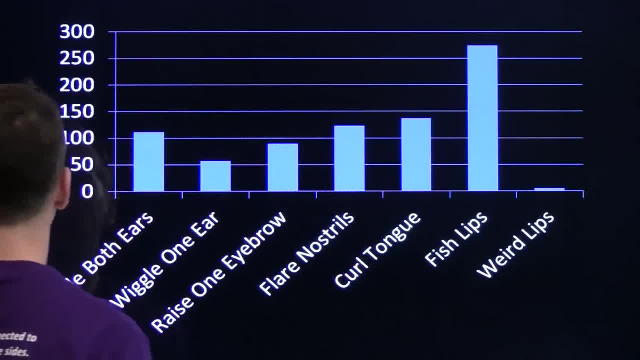 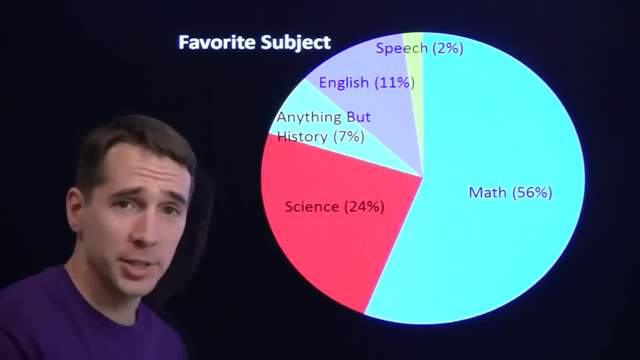 each other. Let's take a look at another type of chart Here. we had another poll of all of our students And we asked them: what's your favorite subject? Now, remember, this is already a problem-solving, so there's some selection bias here. 56% said math And 24% said science, and math is the. 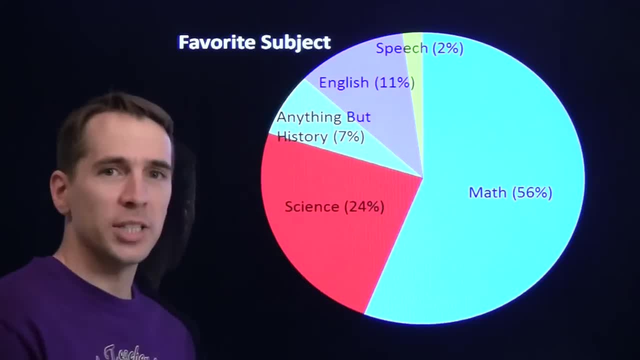 language of science, so that's okay by us. 7% said anything but history. I'm sure math was second there too, so that's okay as well. 11% is English. I can forgive those students. I had some really good English teachers too. 2% said speech, because, well, everybody hates. 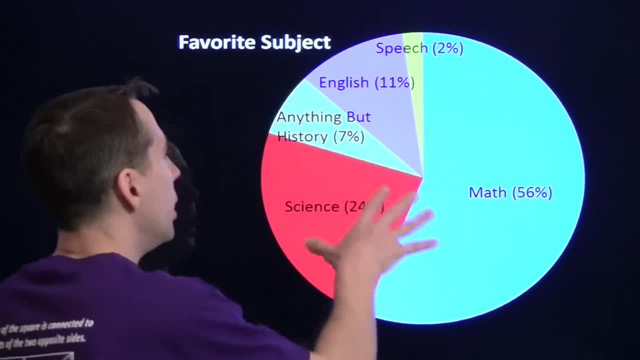 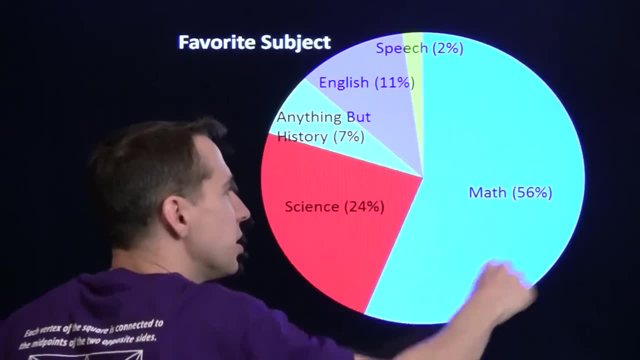 speech. Well, except for me, You know, I love to run my mouth. So this was the result of our poll. Now let's take a look at the results of our poll. Let's take a look at the results of our poll And we draw this nice little pie chart here where each slice of the pie 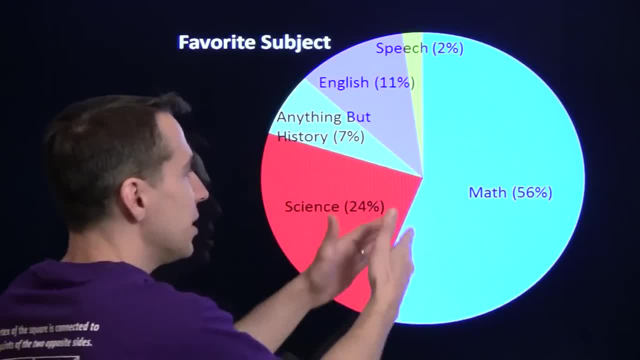 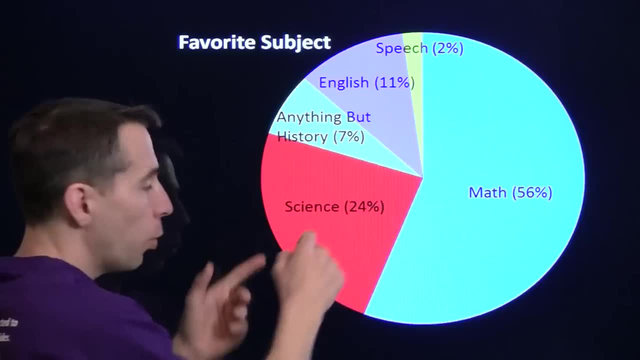 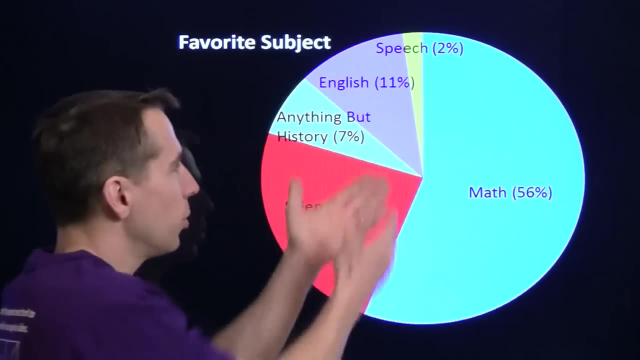 is the size relative to how many people gave that answer. So 56% said math: Slightly more than half the pie is the math slice. 24% said science: Slightly less than a quarter of the pie is science, And same for these. You know, speech. almost no one said speech. It's a. 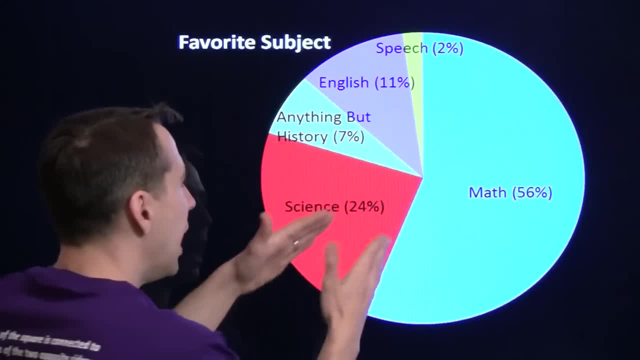 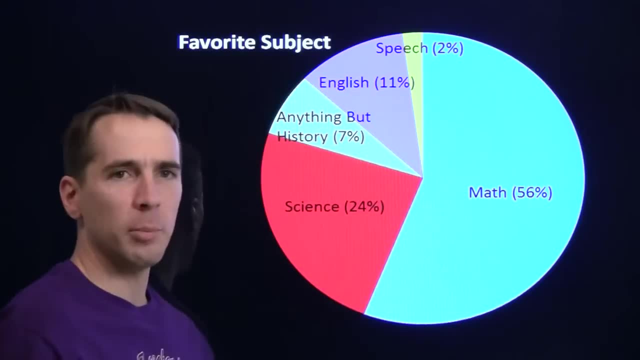 little tiny sliver. So I can tell just by looking at this graph what portion of the whole, without even looking closely at the numbers, I can tell at a glance. a little more than half the people like math, Around a quarter of them like science. Almost nobody likes. 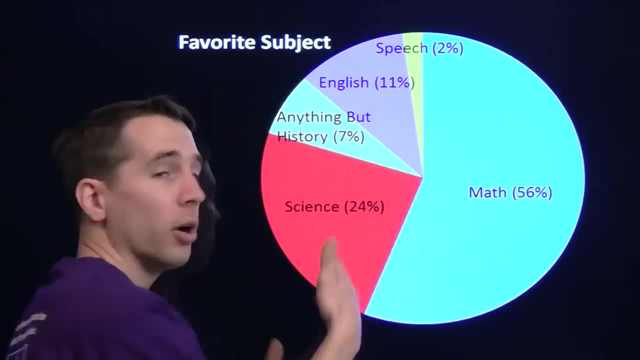 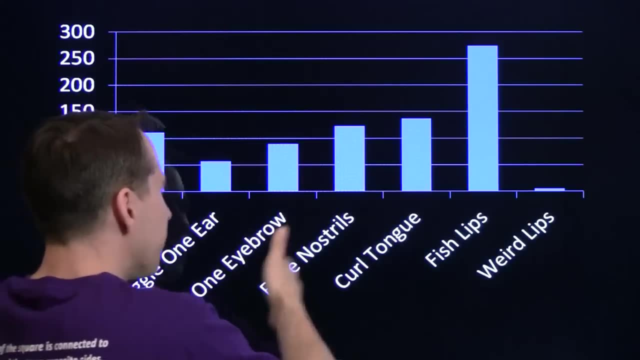 speech- And that's what a pie chart is good for- is revealing parts of a whole, And that's why we're not going to use a pie chart back here. These different skills don't all together make up a whole. Back here, each student is. 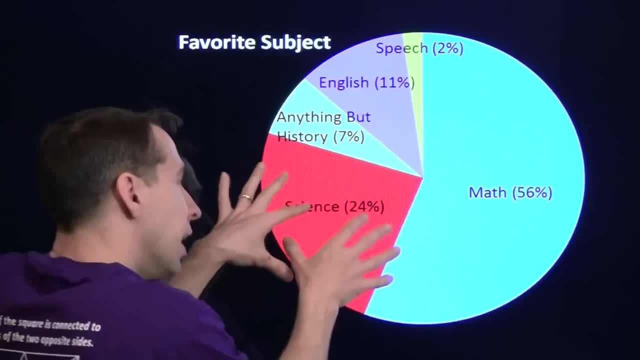 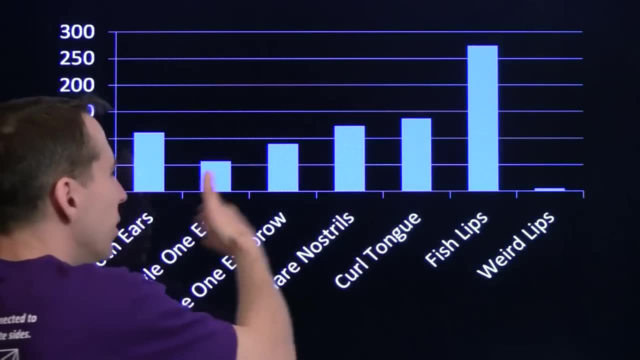 going to fall into exactly one of these slots And all together, when we add all these up, we get all the results, all of the answers to our poll, Whereas over here, some students, some people are going to be in one or two of these, Some of them are going to be done. 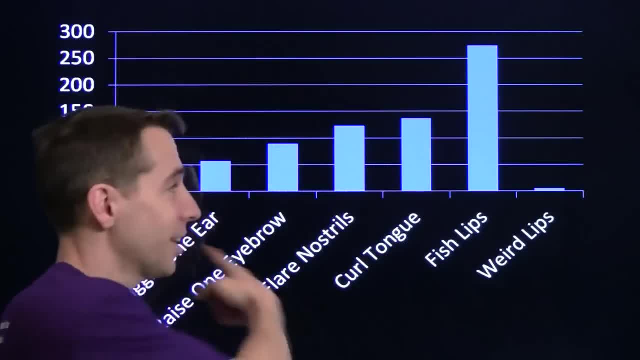 Some people have no skills at all, can't do any of them, And then there are going to be total freaks that can do all seven of them. So we can't put these all together and say that these are all parts of some whole, because some people are in a bunch of these slots. 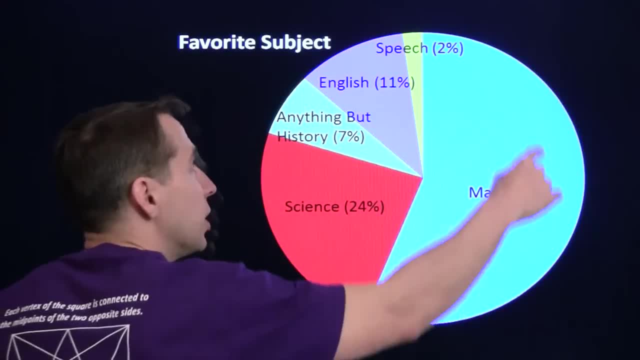 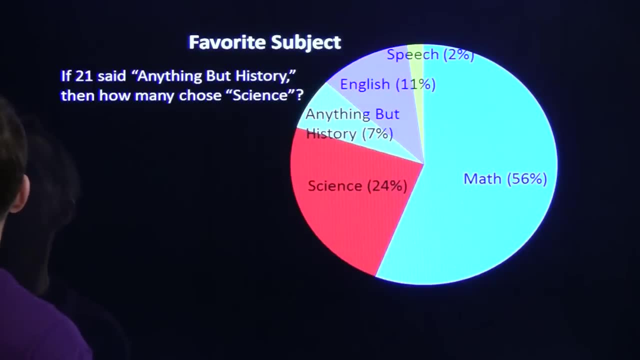 Whereas here each person is in exactly one slot- only one slot. So we can use a pie chart when we want to display parts of a whole, and that's what we're doing Now. let's go ahead and tackle a quick problem using the data here. Imagine 21 said anything. 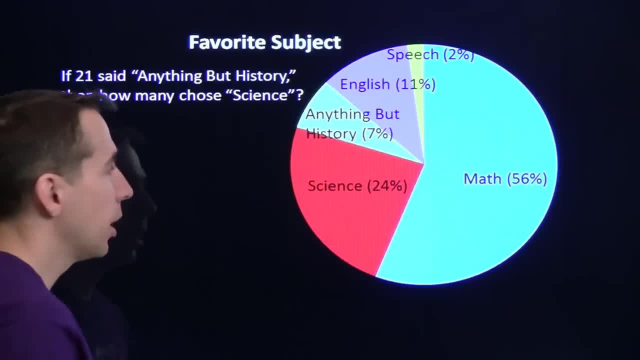 but history? How many chose science? Now we can tackle this problem in a bunch of different ways. First, well, 21 is 7 percent of everybody. So we could just say x is the total and 7 percent of x has to be 21,. so we get an equation. 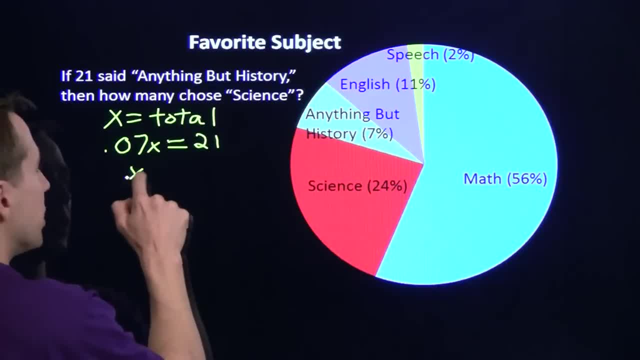 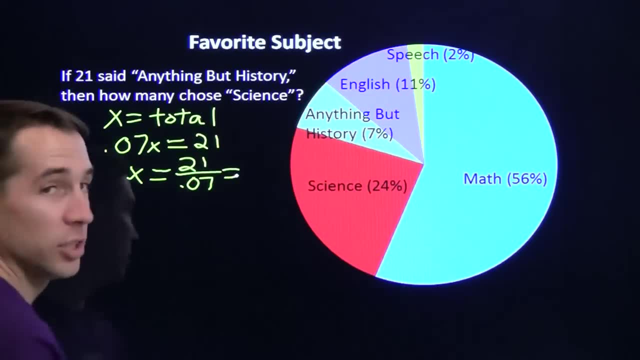 .07x is 21.. .07x, .07x, .07x, .07x equals 21.. Divide both sides by .07.. 21 over .07.. And you divide 7 into 21,, you get 3.. 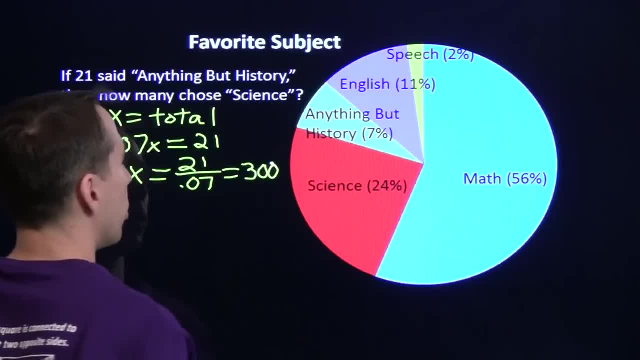 Well, you've got the decimal place to deal with that. It'll come out to be 300.. So once you know that there are 300 total. well, 24% of them said sine. So 24% of 300 is .24 times. 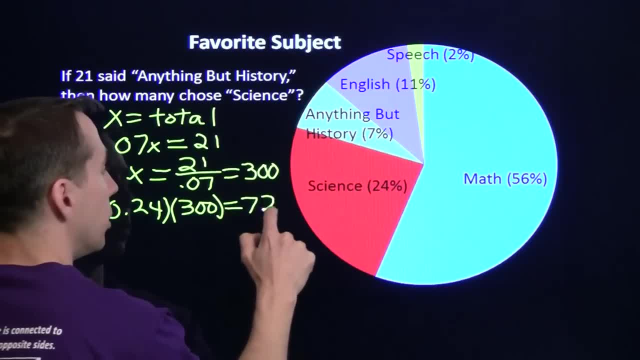 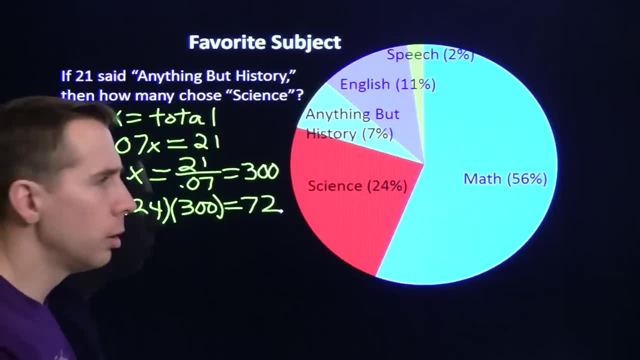 300.. 3 times .24 is 72.. So that's one way we could've tackled the problem. Now, another way we could tackle that is say 7% is 21.. Well, if I divide by 7,, that means 1% is 3.. 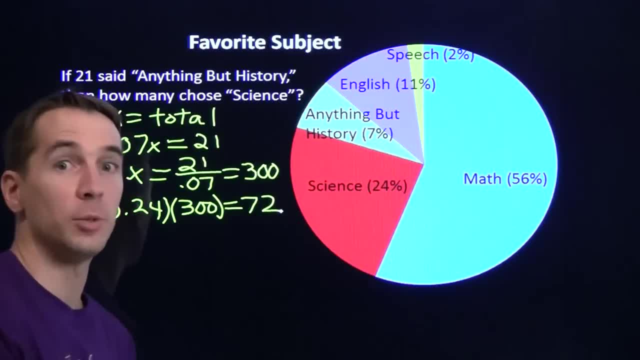 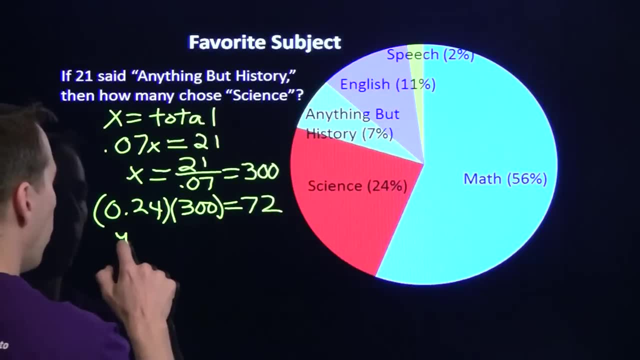 So if 1% is 3, then 24% is 24 times 3.. That gives us 72.. And then yet another way we can do this is we can say: well, y is the number in science, And we can set up .4 timesР, and we can set up .3 timesbb, And then that will give us: 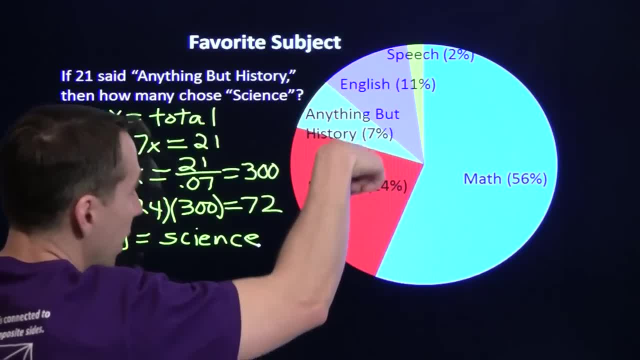 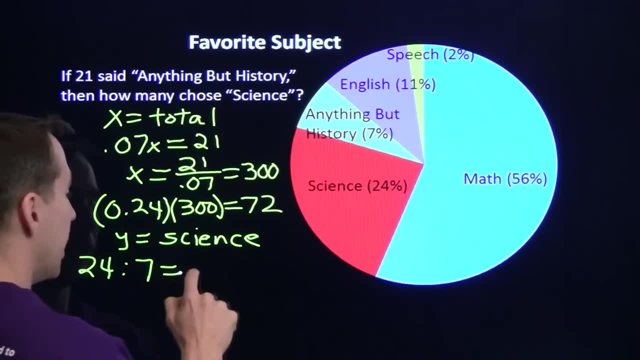 up a ratio here. We know that the ratio of science to anything but history is 24 to 7. And that's going to be equal to y to 21.. Because y is the total number of students in science. we know that 21 said anything but history. So this proportion here comes from our this. 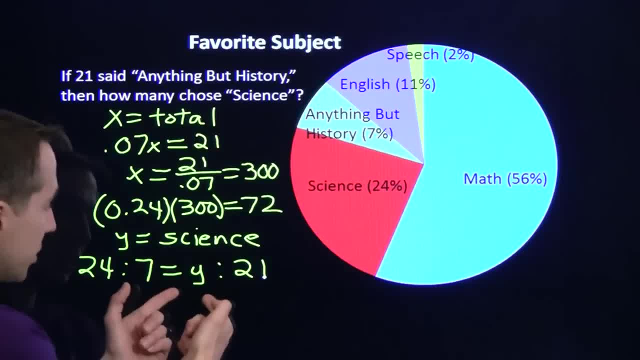 ratio here comes from our percents 24 to 7, and this is the actual number of students, Y in science. 21 said anything but history, And now we can clearly just multiply both parts of this ratio by 3. We'll get 72 again. 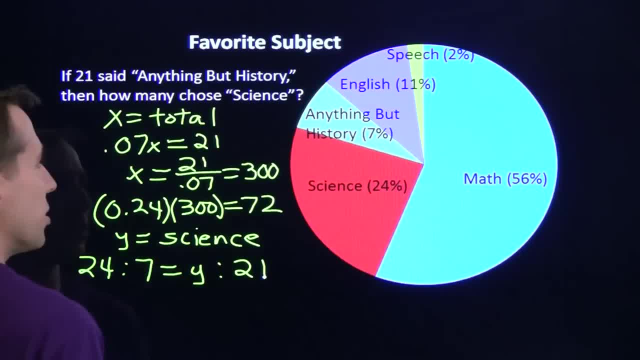 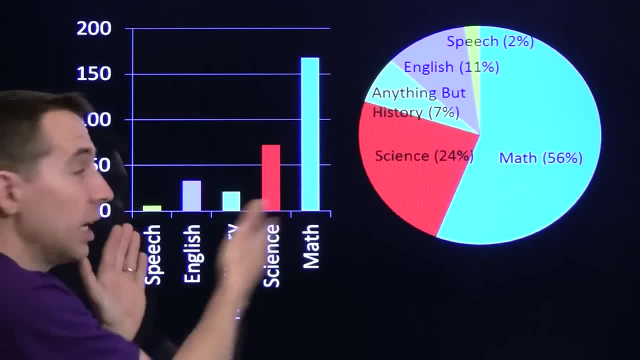 And you might be wondering: why didn't we just show this as a bar chart? And we definitely could. We could have easily taken these the same responses here and stuck them in a bar chart here. Now, what we can't tell from the bar chart is: is math: more or less than half. 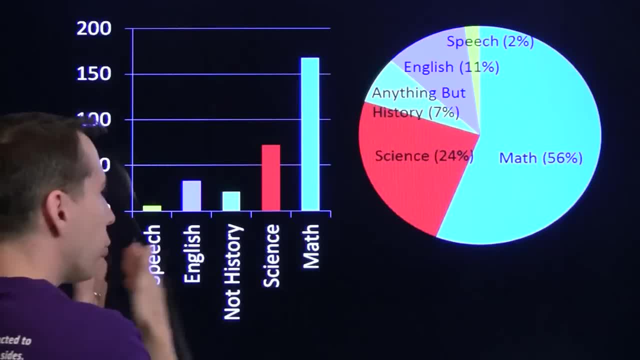 the total. Well, we have to do some thinking here. We can clearly order them using the bar chart, Just like we did with those wicked skills. We can see math was the best, science is the next best, then English, then not history and then speech. But we can't see very easily. 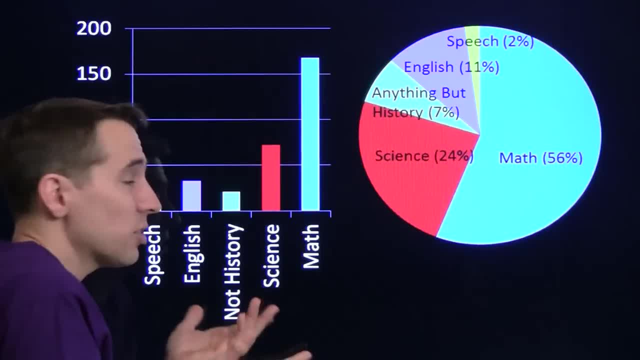 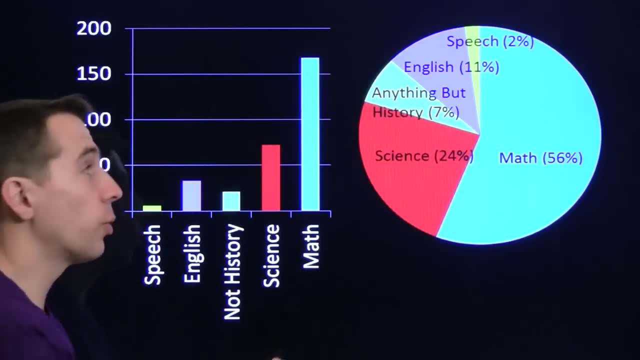 what the proportion of a whole is. We can't see that science actually is about a quarter of the total. The pie chart tells us that. right at a glance We see a little quarter pie slice. We know that science is around a quarter of the total, So the bar chart is: 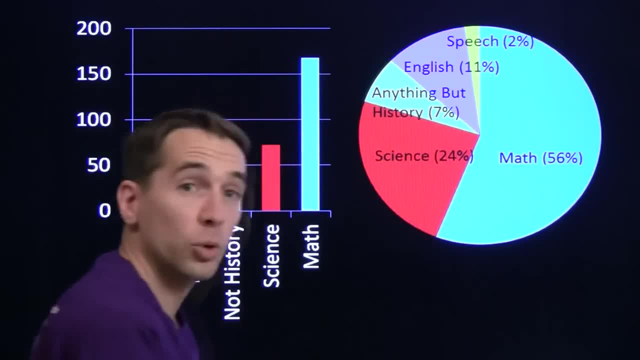 great for us to compare these to each other. The pie chart is great for comparing them to the entire thing. Now that you understand that, we're going to move on to the next part, which is the difference between a pie chart and a bar chart. 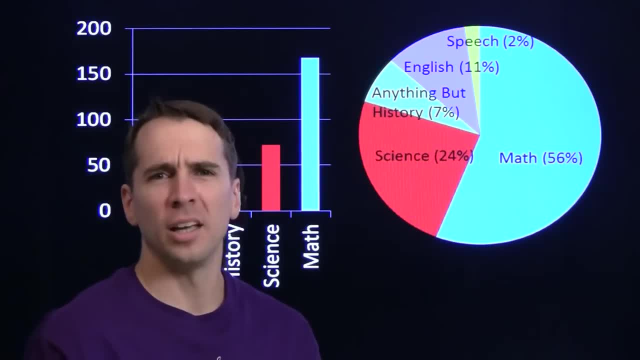 I know exactly what you're thinking. You're thinking: how did he do that weird lip thing?